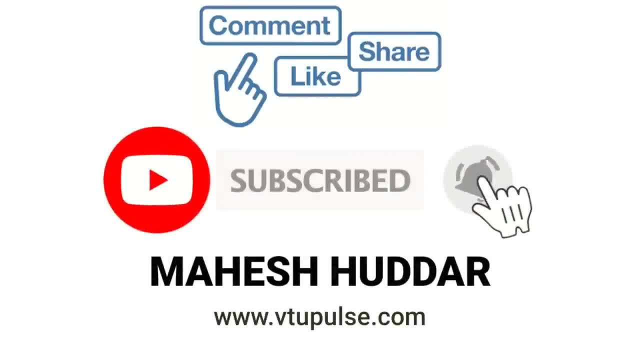 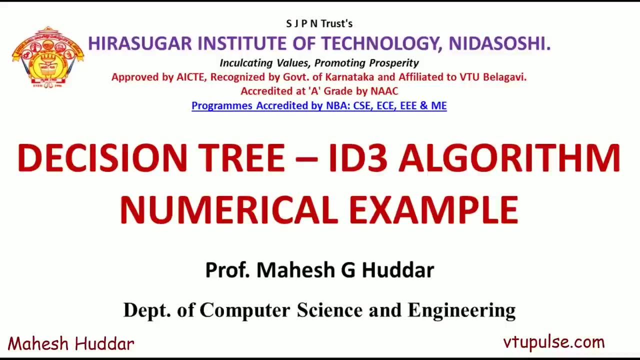 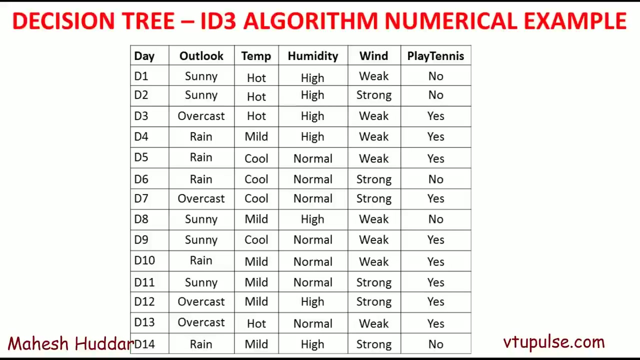 Welcome to machine learning tutorial. In this video, I will discuss how to draw decision tree using ID3 algorithm with a simple numerical example. This is the data set I will be considering for this numerical example. This particular data set contains 14 examples, 4 attributes like outlook, temperature, humidity and wind. 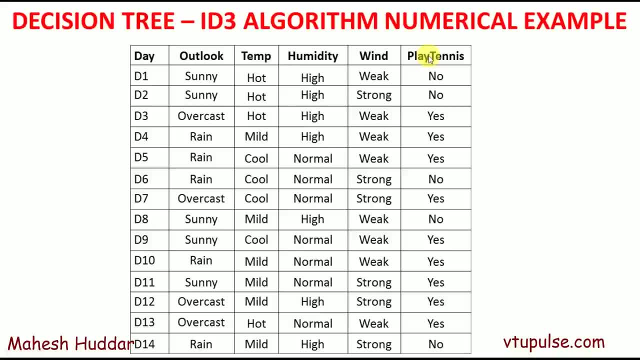 Platinus is the target variable in this case. If you want to draw decision tree using ID3 algorithm, the very first thing what we need to do is we need to understand which is the attribute which is giving the maximum information out of the available attributes. 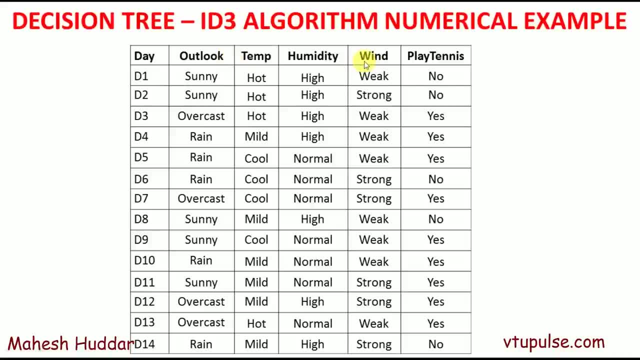 So in this case we have 4 attributes. Out of 4 attributes, we need to draw the maximum information. We need to calculate the information gain of every attribute. The attribute which is having the maximum information gain will be considered as a root node. 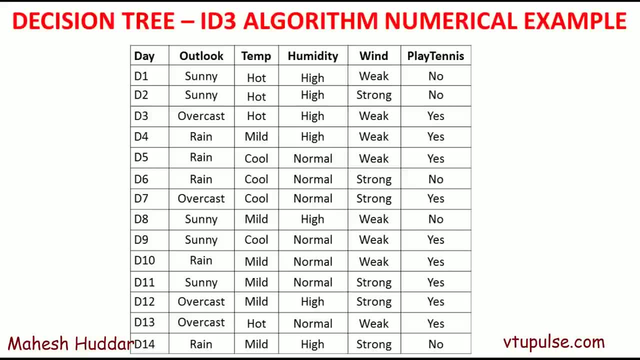 And then we will start building the tree here. So what we do initially is we will try to calculate the information gain of each and every attribute in this example. So first we will consider the first attribute. So the attribute name in this case is outlook. 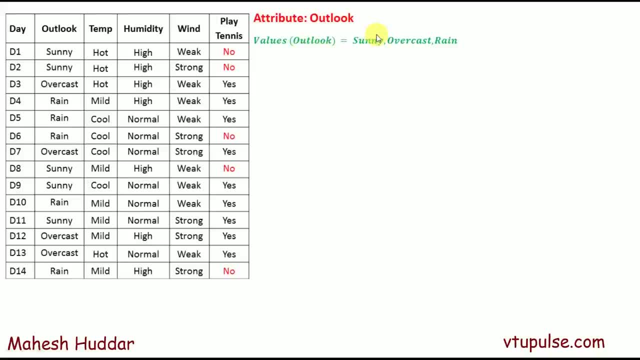 And the possible values of outlook are sunny, overcast and rain. If you want to calculate the information gain of every attribute, the very first thing we need to do is we need to calculate the entropy of the whole data set and the entropy of individual attribute values. 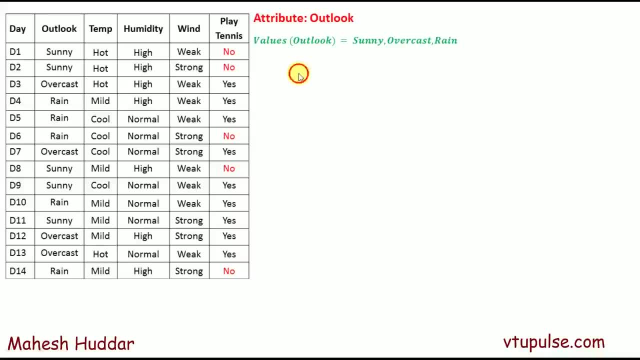 So the entropy of entire data set is calculated something like this. So the whole data set is represented as S. In this particular data set we have 9 positive examples and 5 negative examples. So the negative examples I have marked as red. 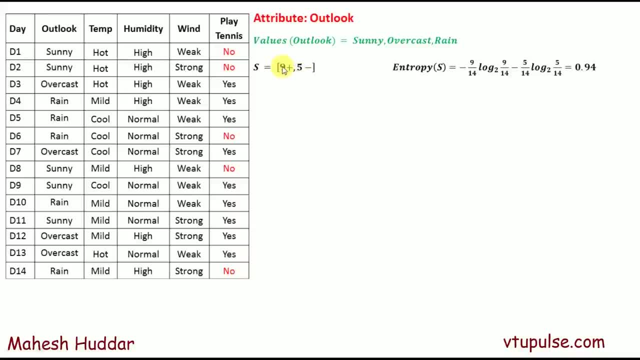 There are 5 negative examples and 9 positive examples. So the entropy of this whole data set S is equivalent to minus proportion of positive examples, That is, 9 divided by 14. here Log 9 divided by 14 to the base 2 minus proportion of negative examples. 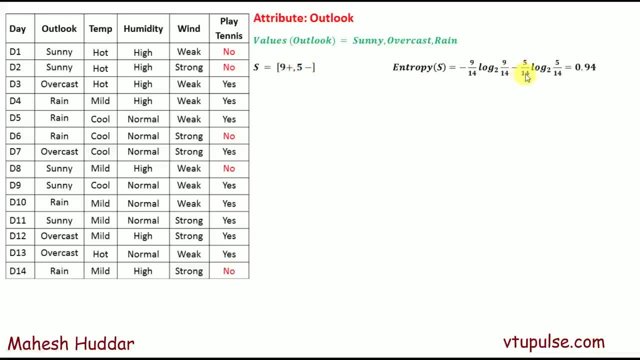 That is, 5 divided by 14.. So 5 divided by 14, log 5 divided by 14 to the base 2, which is equivalent to 0.94.. So this is the entropy of entire data set. Similarly, we need to find the entropy of sunny. 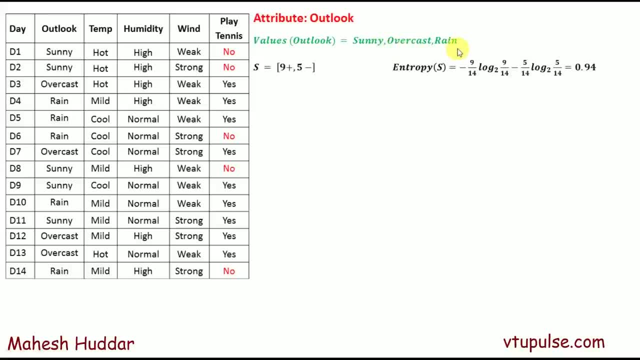 entropy of overcast and then entropy of rain here. So the S sunny, that is. we need to consider the data set, which is consisting of sunny for outlook. So how many examples are there? We need to count. So, first and foremost thing, 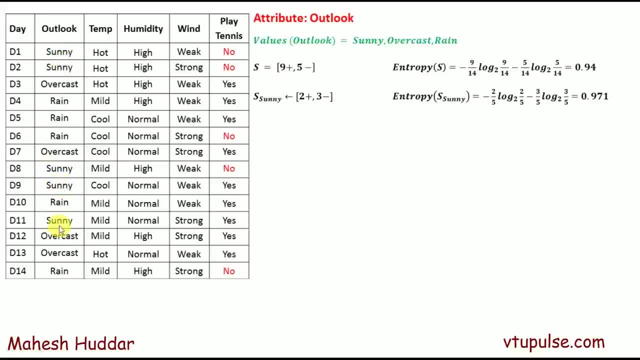 1,, 2,, 3,, 4, 5.. 5 examples are there Out of 5, how many positive and how many negative We need to count. So first one is negative. Second one is negative. Third one is negative. 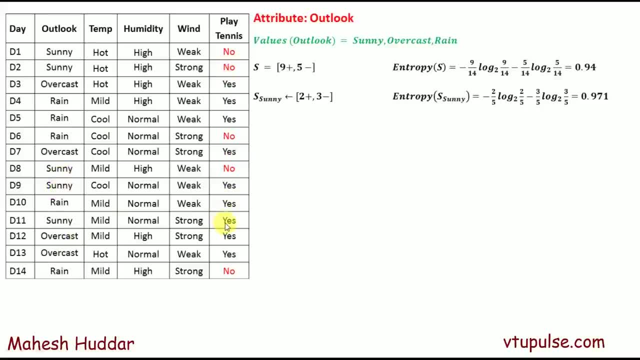 Fourth is positive and fifth one is positive. So 2 positive examples we have and then 3 negative examples. So the entropy of S sunny is equivalent to proportion of positive examples, That is, 2 by 5, log 2 by 5 to the base, 2 minus proportion of negative examples. 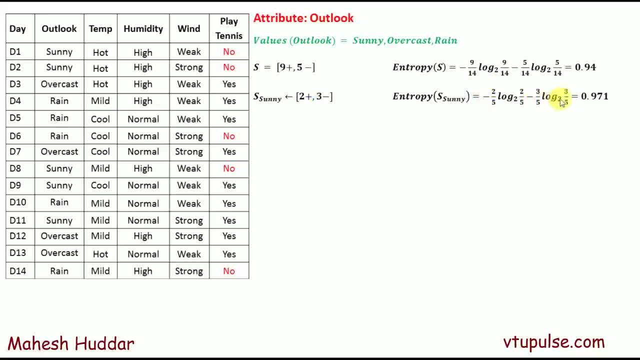 That is, 3 by 5. log 3 by 5 to the base 2, which is equivalent to 0.971 in this case. Similarly, we need to find the entropy of overcast, entropy of rain here. So for overcast. 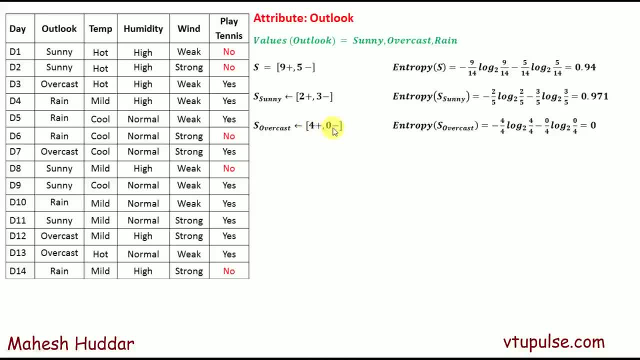 we have 4 positive examples and 0 negative examples. If you have only positive examples or only negative examples for particular value in the given data set, the entropy is always equivalent to 0. So there is no need to calculate this particular part. 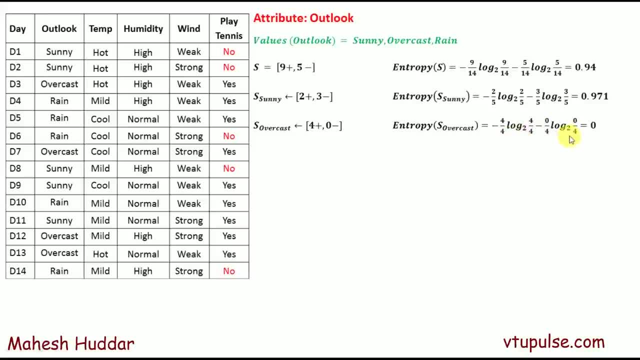 but this is the first time, So I have written the formulae, but we can directly write the value as 0 here, That is, if you have only positive examples or only negative examples. So in this case we have only positive examples, it is equivalent to 0.. 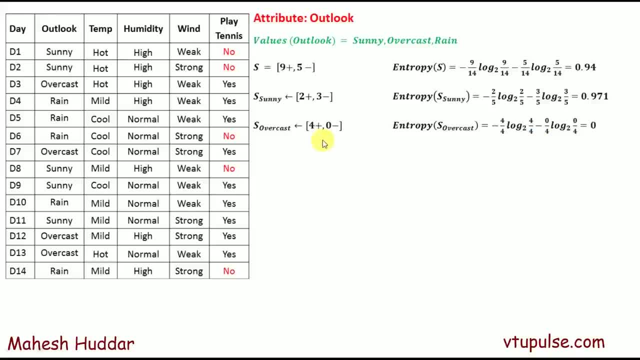 Sometimes what happens is we may have equal number of positive and negative examples. The entropy is always equivalent to 1.0 in that case. So that is also we can directly write. So we will come across such examples at the later stage. Similarly, 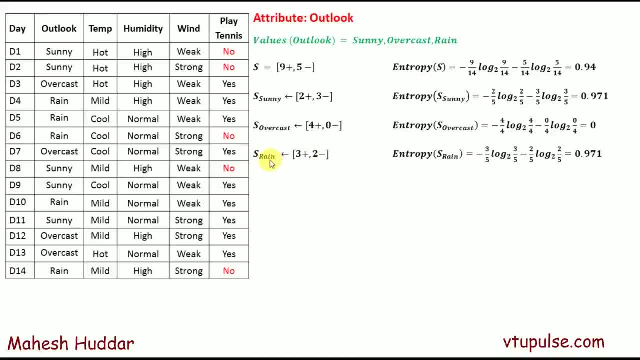 S rain. there are 3 positive examples, 2 negative examples. Entropy of rain is equivalent to proportion of positive and negative examples. S rain is equivalent to proportion of positive examples- log proportion of positive examples to the base 2.. Proportion of negative examples- log proportion of negative examples to the base 2,. 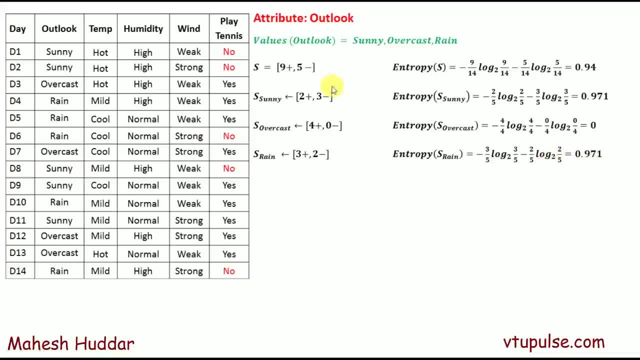 which is equivalent to 0.971 here. So we have calculated the entropy of entire data set, entropy of individual values of this particular outlook attribute. Now we need to calculate the gain. So the gain formula is gain outlook given this particular data set S. 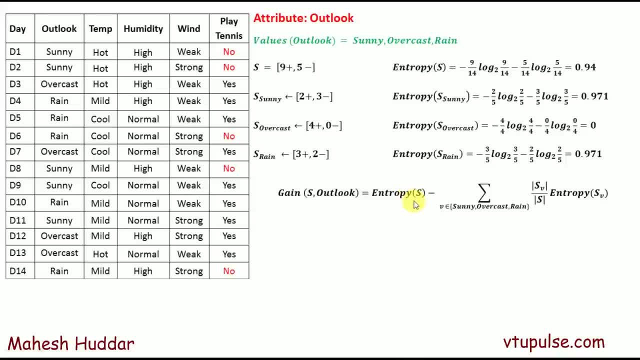 which is equivalent to entropy of whole data set, that is, entropy of S minus summation of cardinality of SV divided by S. cardinality of S, that is SV, is nothing but what? the number of possible values of sunny, overcast and rain. 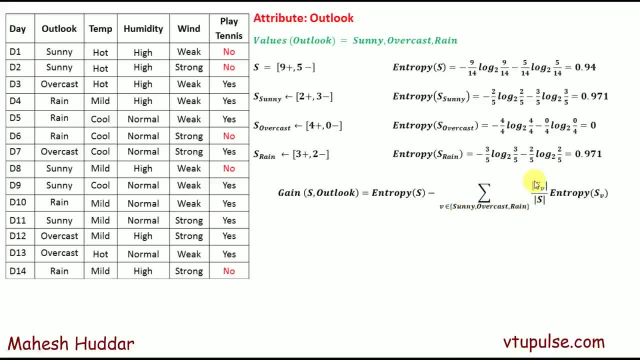 So first time it is sunny, second time overcast, third time rain. So S sunny divided by S S overcast, divided by S S rain, divided by S here And entropy of that particular attribute value, First time it will be sunny. 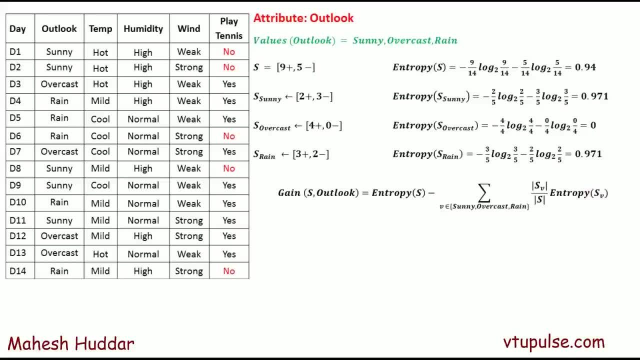 second time overcast, and third time it will be rain in this case. So if you expand this particular thing, you will get something like this. So gain of outlook with respect to this S is equivalent to entropy of S as it is. 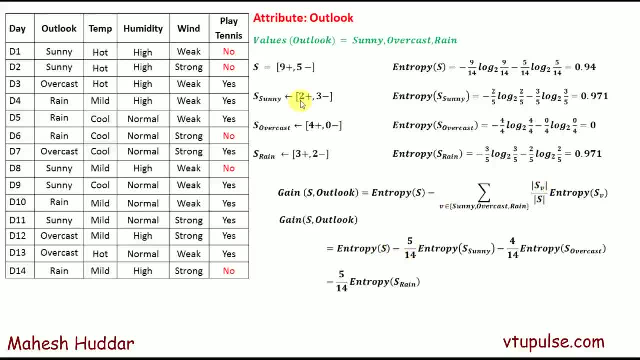 So how many number of times the first one, sunny, is appearing? 2 plus 3, that is 5 times it is appearing. Total number of examples are 14.. So 5 by 14, entropy of S sunny minus. 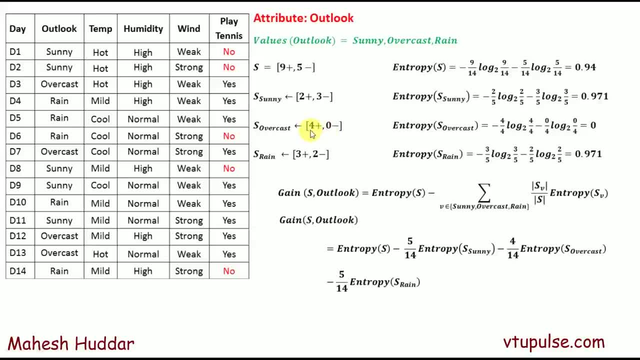 this minus will be as it is. How many number of times overcast is coming? It is 4 times 4, divided by 14, entropy of S overcast here, minus 5 by 14, entropy of S rain here. 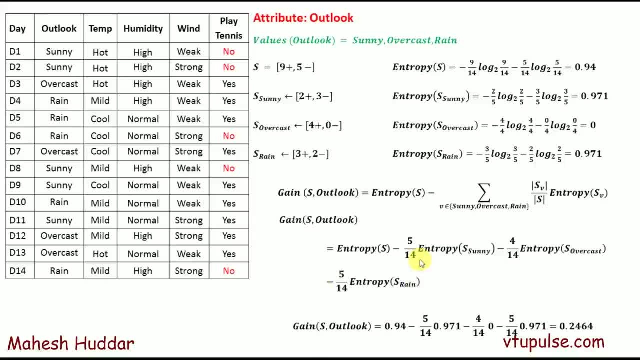 So if you put the values of all the entropies, we will get the final answer as 0.2464.. So this is the information gain of outlook attribute. Similarly, we need to calculate the information gain of remaining 3 attributes. 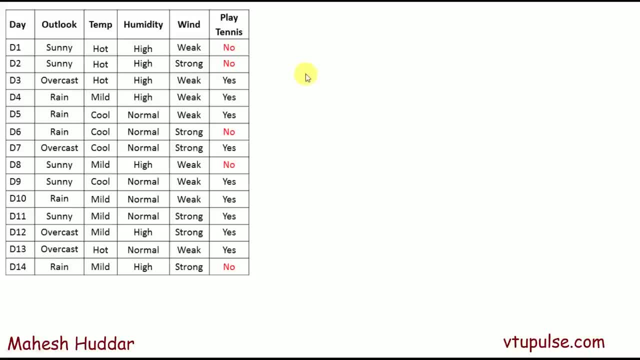 So the next attribute is temperature. So I will name attribute as temperature. The values of temperature are hot, mild and cool. So those are the things were listed here. First we need to calculate the entropy of whole data set, which will be same because the same thing has been done for outlook. 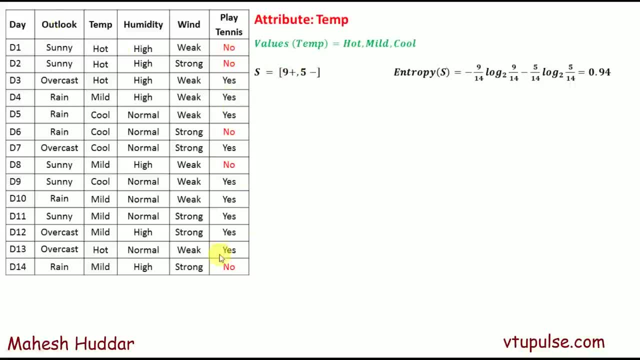 There are 5 negative examples are there and 9 positive examples are there, which is equivalent to 0.94.. Entropy of hot hot is appearing 4 times. You can see here: 1,, 2,, 3, and then it is 4 times. 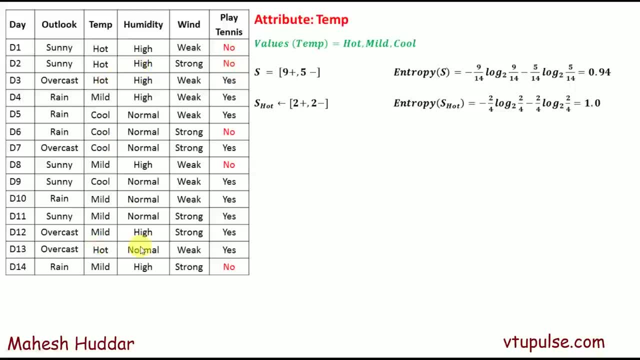 So first 2 are negative and third one is positive and fourth one is positive. So there are 2 positive and 2 negative examples. So the entropy of S hot is equivalent to 1.0 directly, So there is no need to calculate it. 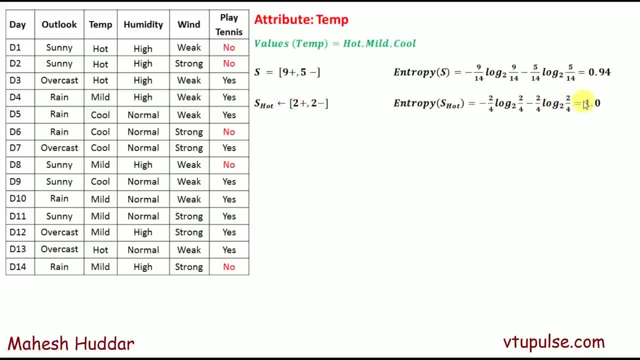 If the number of positive and negative examples are equal, the entropy is equivalent to 1.0.. Similarly, we can calculate the entropy of mild. The mild is appearing 6 times. 4 are positive and 2 are negative. in this case, 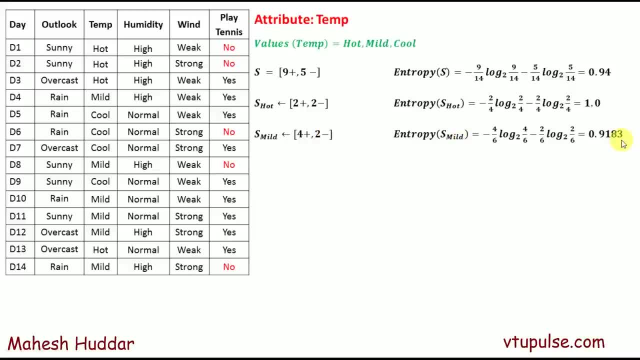 The entropy of S mild is equivalent to 0.9183.. Similarly, entropy of S cool is equivalent to 0.8113.. In this case, we have 3 positive and 1 negative example. here, Similarly, we use the gain formulae. 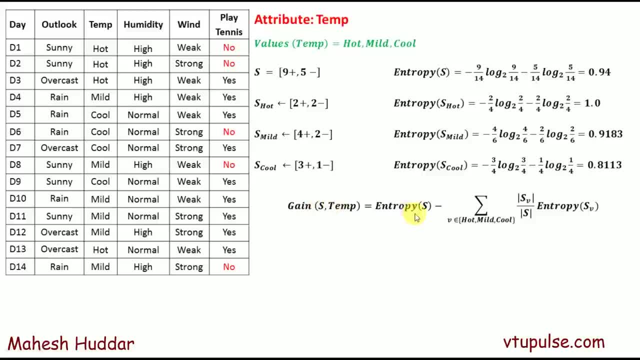 gain of temperature with respect to S, which is equivalent to entropy of S minus. In this case, these are the 3 values: hot, mild and cool. So S hot divided by S. entropy of S hot minus. S mild divided by S. 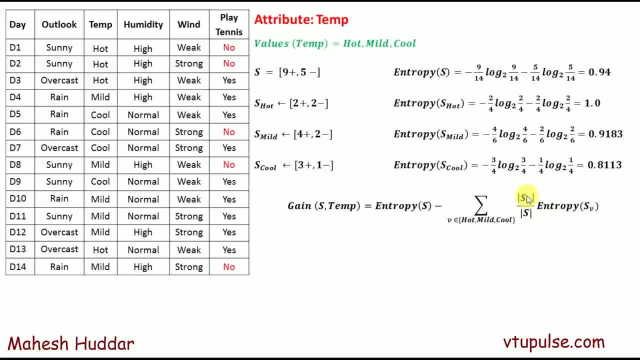 entropy of S mild. And the third time it will be cardinality of S cool divided by cardinality of S entropy of S cool. So if you put those particular values, the gain of temperature with respect to S is equivalent to entropy of S minus 4 by 14.. 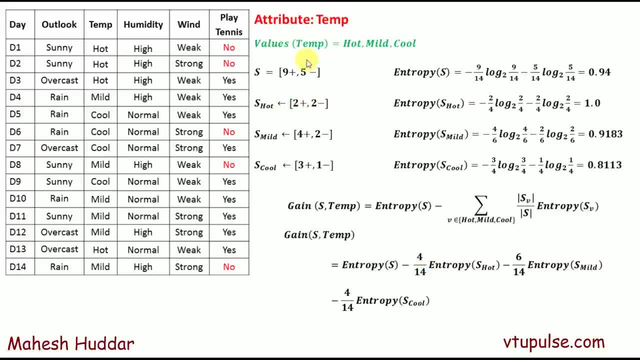 That is the number of time hot is appearing. It is appearing 4 times out of 14.. So 4 by 14, entropy of S hot minus the number of times mild is appearing, 4 plus 2, that is 6.. 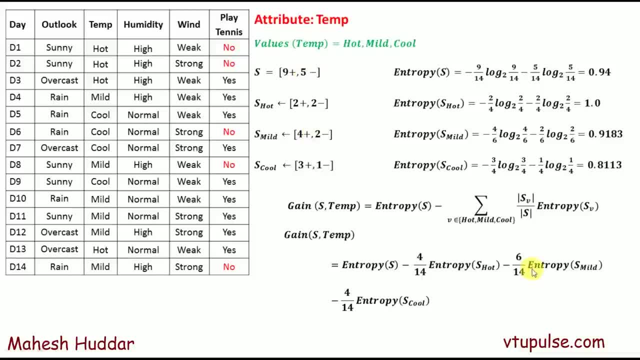 6 divided by number of times out of 14.. So 6 divided by 14, entropy of S mild. And the third one is cool. So 3 plus 1 is 4,, 4 divided by 14, entropy of S cool. 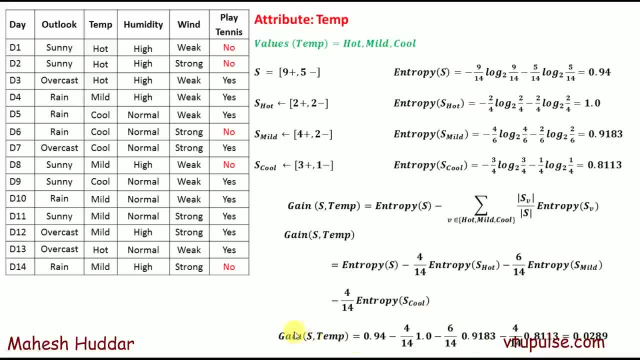 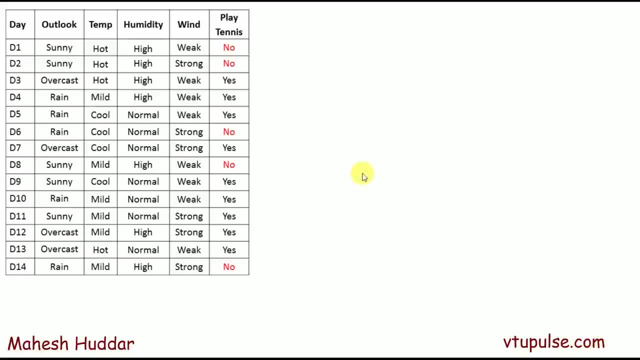 So if you put the values of entropy, we will get the gain of temperature with respect to S, which is equivalent to 0.0289.. Similarly, we need to calculate the gain for the next attribute, that is, humidity. I think there are two possibilities for humidity. 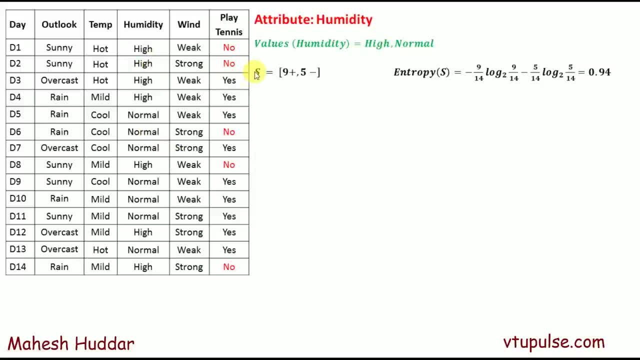 One is high and another one is normal. The entropy of entire data set is 0.94.. Entropy of S high, that is, S high is appearing 7 times. Out of that, 3 are positive and 4 are negative. 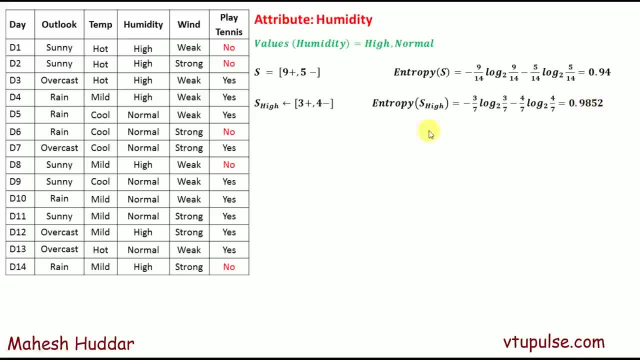 So the entropy is 0.9852.. Similarly, S normal. it is appearing 7 times again. 6 are positive, 1 is negative. So the entire entropy of S normal is equivalent to 0.5916.. Gain of humidity with respect to S is: 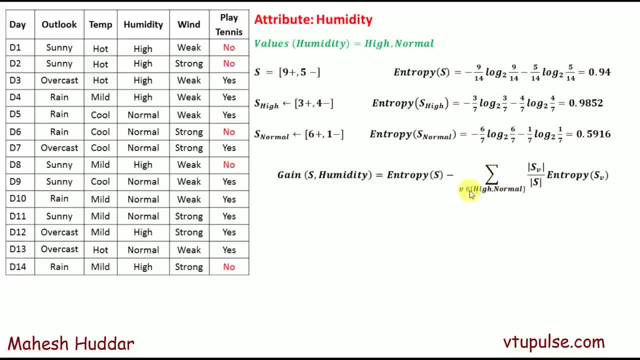 entropy of S minus. in this case the values are high and normal. We need to put it over here. So the gain of humidity with respect to S is entropy of S minus 7 by 14, because 7 times high is appearing. 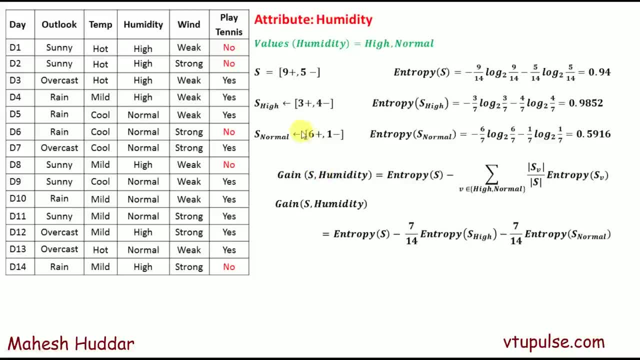 So 7 by 14, entropy of S high and normal is appearing 7 times again. So 7 by 14, entropy of S normal. Put the values of entropy, you will get the final answer as 0.1516.. 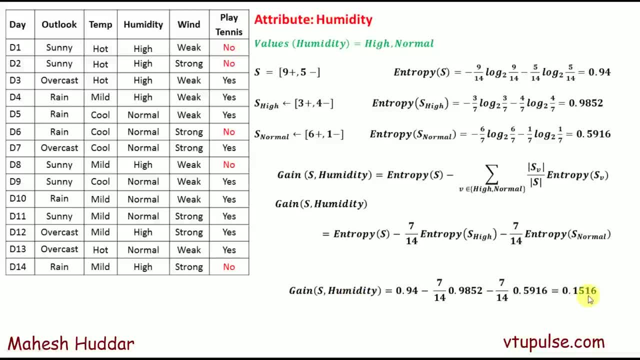 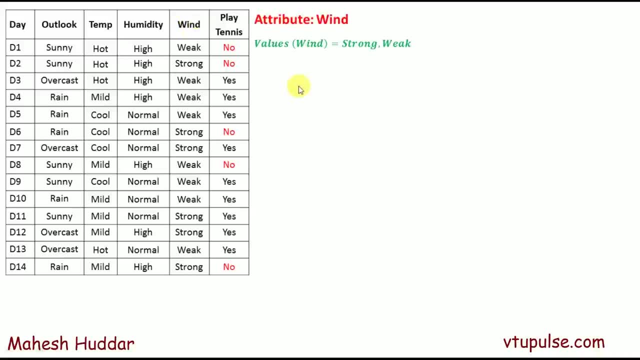 So this is the gain of humidity in this case. Similarly, we need to calculate the information gain of the last attribute, that is, wind. I have given those calculations here. You just follow the calculation, you will understand it. Pause the video for a minute. 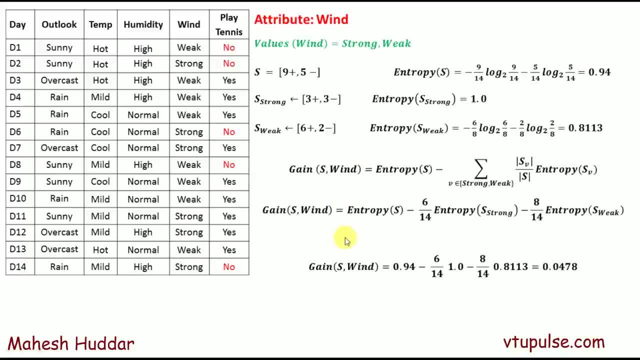 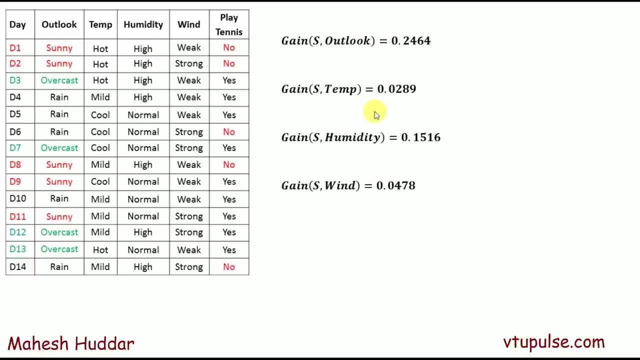 and then check your calculations. In this case we got the gain of wind is equivalent to 0.0478.. Once you calculate the gain of every attribute, we need to check which attribute has the maximum information gain. So if we compare all four gains in this case, 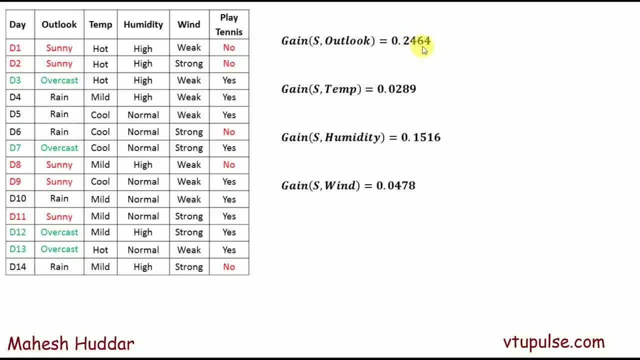 the outlook is having the maximum gain, that is 0.2464.. So we will consider outlook as the root node in this case. So now, once you consider outlook as a root node, how many possibilities are there for outlook? we need to check. 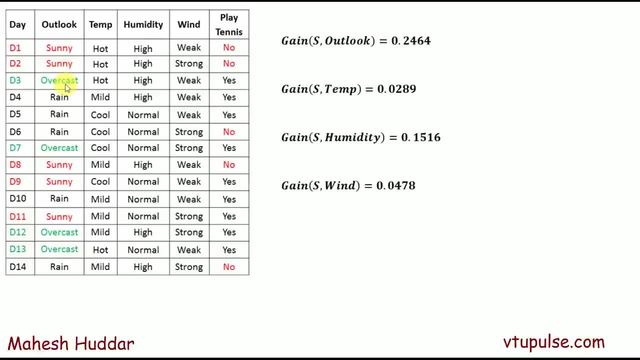 The first possibility is sunny, second one is rain, overcast, and the third one is rain here. So the root node is overcast outlook. So we need to draw three branches: One is for sunny, second one is for overcast. 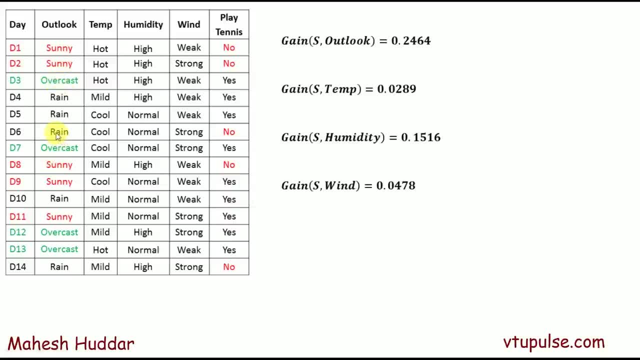 and third one is for rain here. So that's the one thing we need to remember. And the second thing is: whenever I consider outlook is equivalent to sunny, we have only five times sun is appearing, So that is in D1,, D2,. 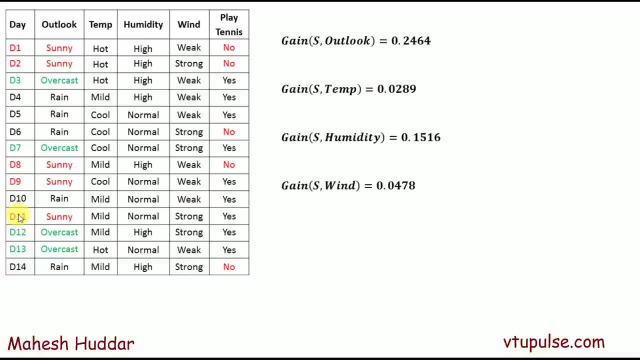 D8,, D9, and D11.. Only these five examples we need to consider. When it comes to overcast, we need to consider D3,, D7, and D13.. When it comes to rain, we need to consider D4,. 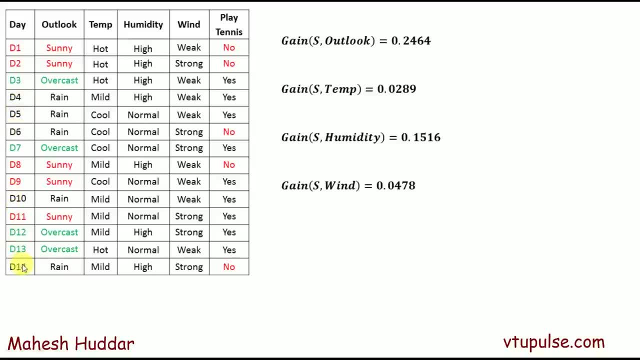 D5,, D6,, D10, and D14 in this case. So these are the things we need to consider. And one more thing we need to notice here: whenever I consider sunny as one branch, what is the target variable? So here, 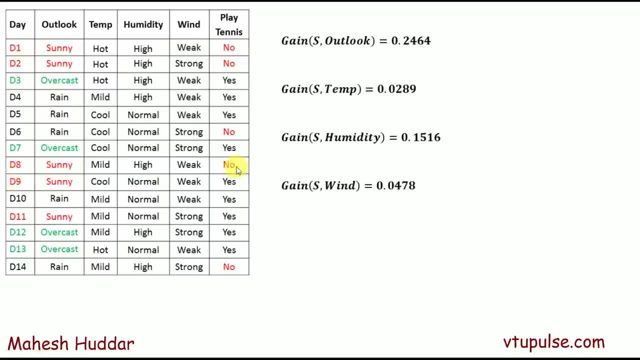 D1, D2 are no, D8 is no, D9 is yes. So, and one more thing is, D11 is also yes. So out of five, I think, three are negative and two are positive, So we cannot say that whether we need to put yes or no over there. 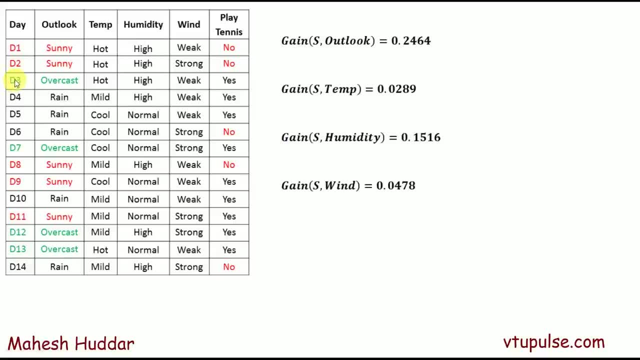 So that's the one thing we need to understand. Similarly, for overcast: if you look at the overcast, overcast is having positive here, overcast is having positive. here. overcast is having positive. here, overcast is having positive. 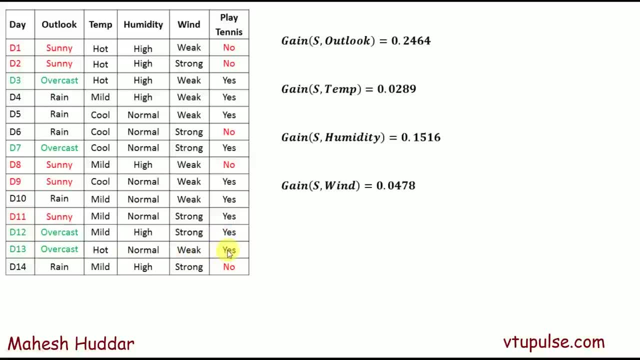 that is yes. So in all the four examples we have yes, So we can directly write yes in that case. Similarly for rain: the first one is yes, second one is yes. you can see here: D6 is no, D10 is yes. 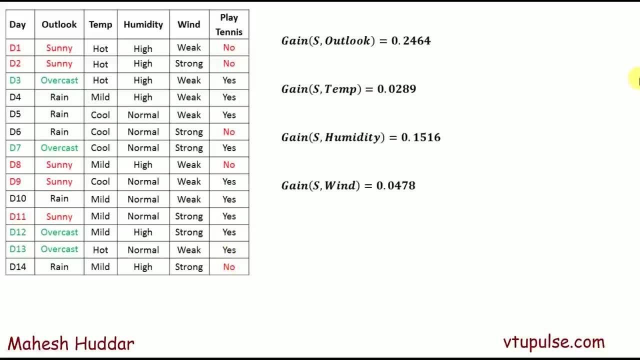 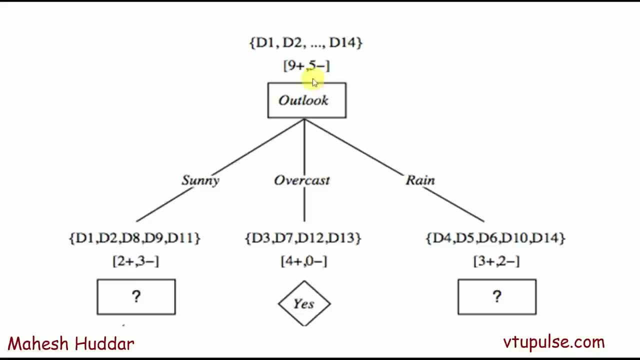 D11 is again no, So it is having positive here, So it is having combinations of yes and no, So we cannot write yes or no directly there. So this is how actually the tree looks like Initially: we need to write the outlook as the root node. 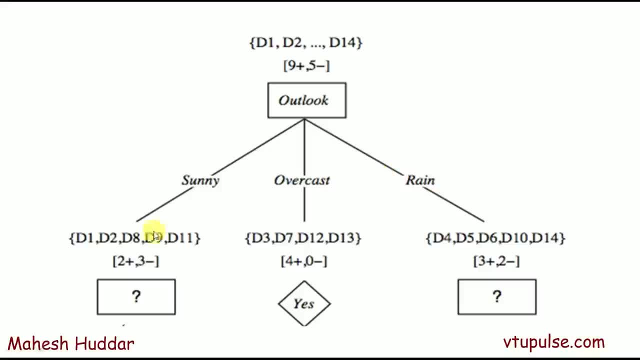 There are three branches. This is the sunny, overcast and rain. These are the examples where sunny is present. These are the examples where overcast is present And these are the examples where rain is present, As I said earlier, when it is the sunny. 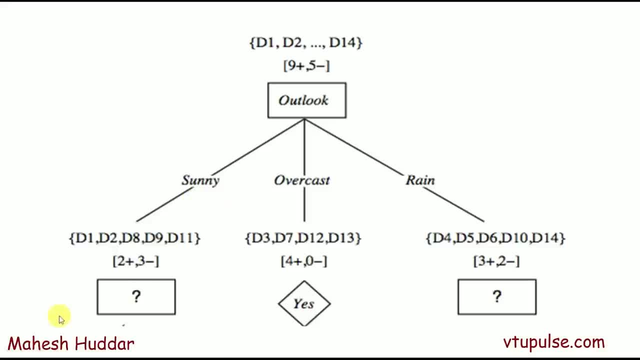 we have two examples which are positive And three are negative, So we cannot write yes and no as a label here, Because it is a combination of positive and negative here. But when it comes to this overcast, all four examples are positive. 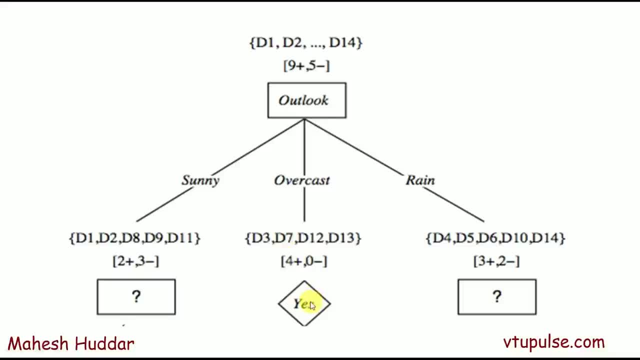 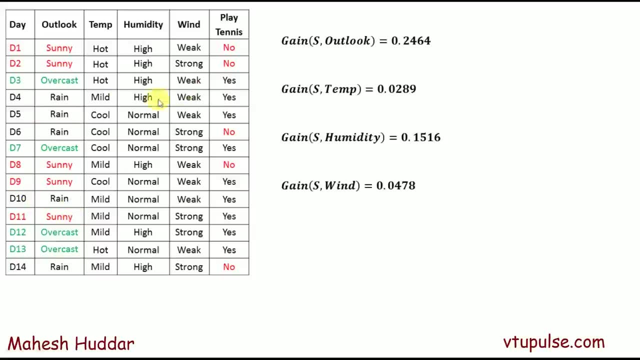 So directly we write yes here. This is a leaf node or we got the answer here. And when it comes to rain, we have three positive and two negative, As I have shown in this particular case, Rain. first one is yes, second one is yes. 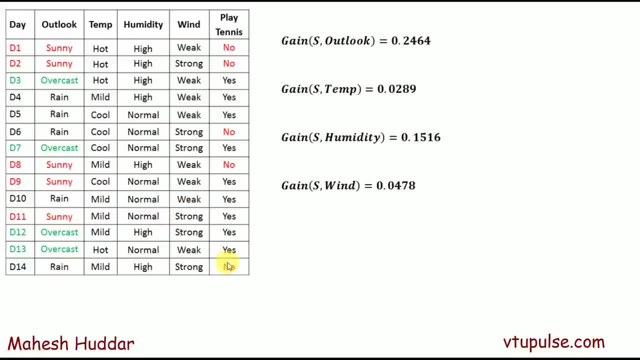 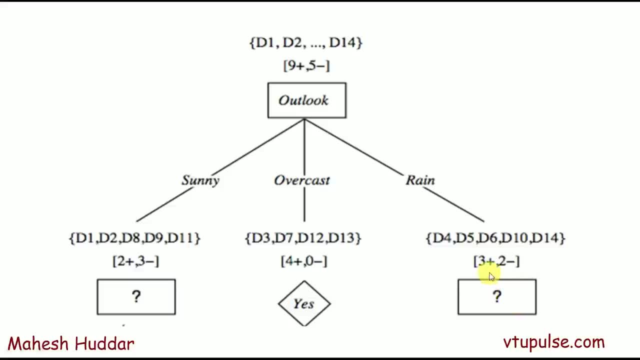 third one is no, fourth one is yes and fifth one is no. So there are three yes are there and two no are there. Again, we cannot write any label here like yes and no, Because we have a combination of yes and no as the examples in this case. 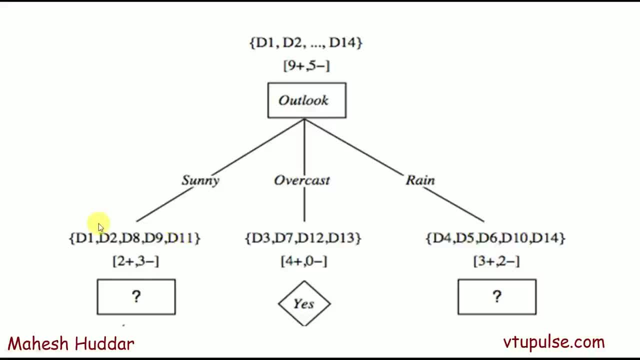 So what we need to do is we need to consider these five data points or the examples, And then we need to consider which attribute should be written here, That we need to do the calculation Similarly over here. These are the five attributes we need to consider. 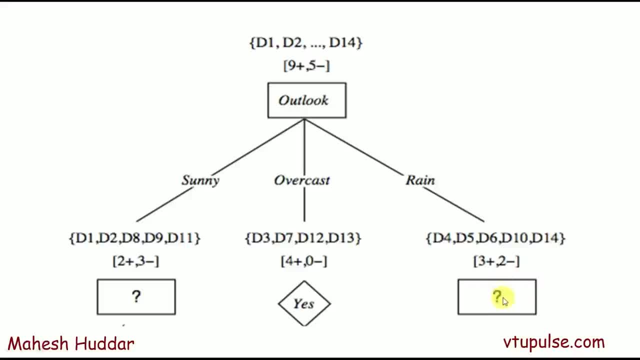 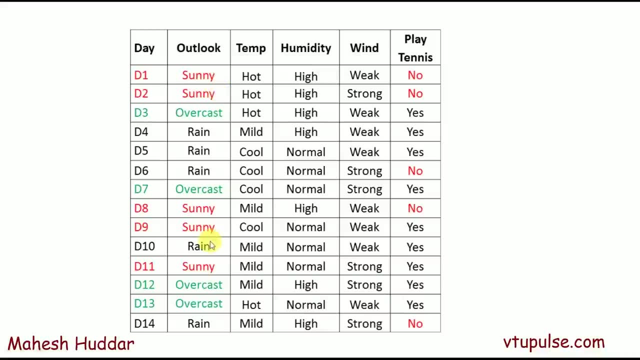 And then we need to calculate the attribute which is having the maximum information gain on the right hand side. So we will continue from this side. These are the total 14 examples are there From this particular total 14 examples on the left hand side. 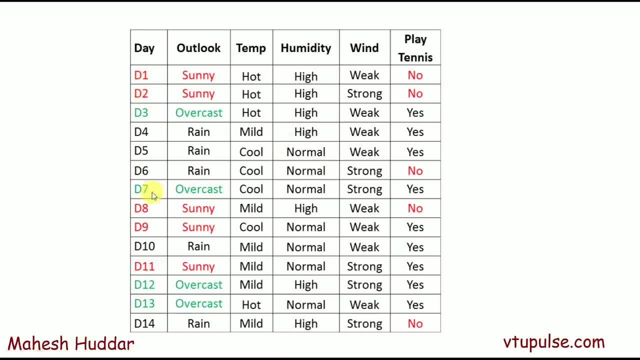 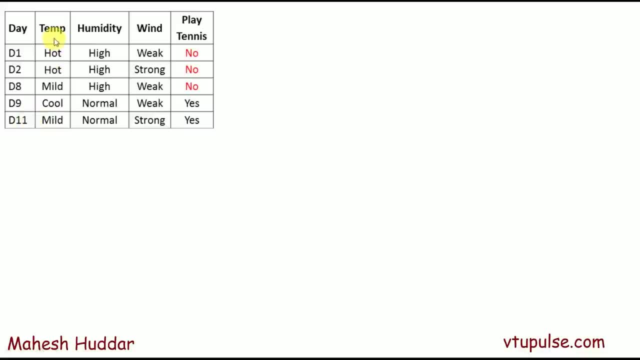 On the left hand side we have sunny, So D1, D2, D8, D9 and D11.. Only five examples should be considered. So I have considered only those particular five examples- Temperature, humidity and wind- Because outlook is already considered. 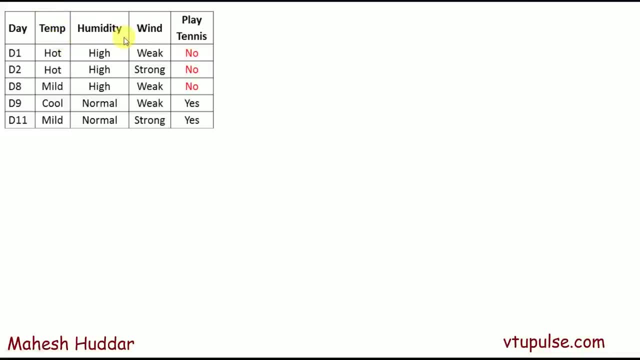 So we don't need to consider outlook. So only three attributes are remaining Out of five. three are negative examples and one is two are positive examples. Again, what we need to do is we need to calculate the gain of all three attributes. 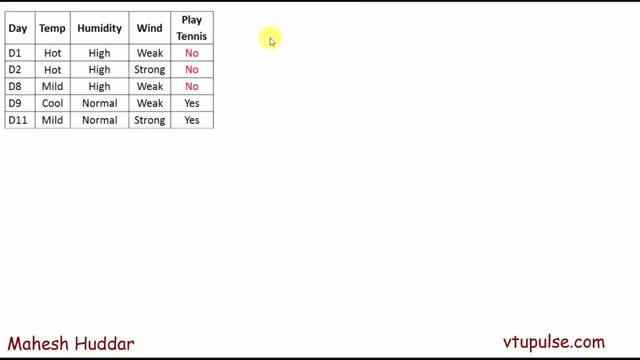 And then we need to build the tree. So I will consider the first attribute, That is, temperature, In this case that values of temperature are hot, mild and cool, And the entropy of this particular data set, that is. five examples are there. 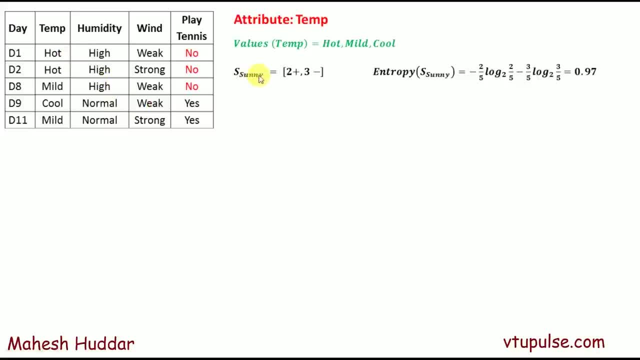 So how did you got this? particular five examples is: whenever we have the outlook is equivalent to sunny. So that's the reason. yes, sunny is equivalent to three negative are there and two positive. That is two plus three minus, And the entropy of this one is: 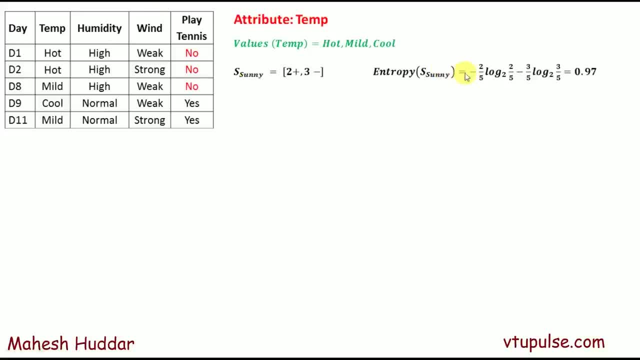 entropy of S sunny, That is, this particular data set is equivalent to proportion of negative, positive examples And then proportion of negative examples. Put this particular values over here. you will get the entropy as 0.97.. Now entropy of this hot. 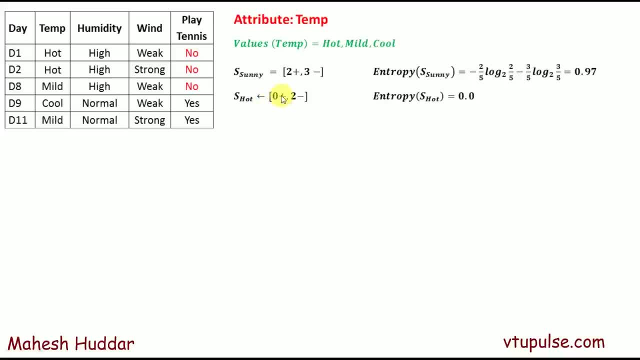 mild and cool. we need to calculate. So S hot there are, we can see here there is a hot is appearing two times. Both of them are negative examples. So zero plus two minus, Because only negative examples are there. 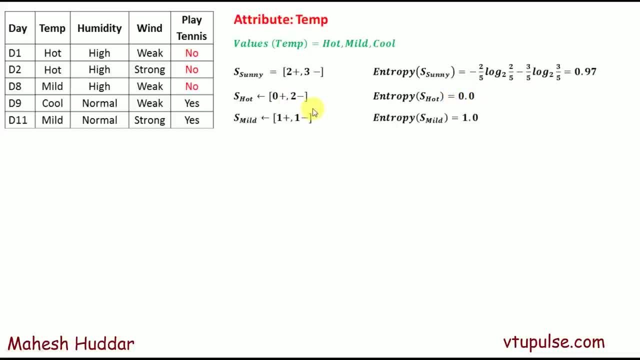 the entropy is zero. Similarly for mild- if you see mild here- this is one is no, another one is yes, one is positive and one is negative. Because equal number of positive and negative examples are there- the entropy is equivalent to 1.0.. 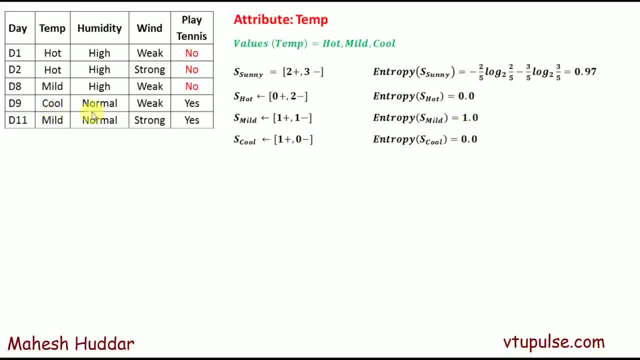 When it comes to the next one, cool, we have only one example that is also yes. So one plus, zero, minus. Because only positive examples are there, the entropy is equivalent to zero in this one, So use this particular gain formulae. 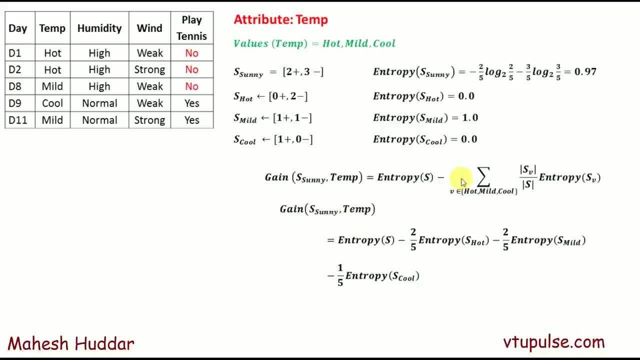 that is again the same procedure. we need to follow The gain of temperature with respect to S sunny: entropy of S sunny here. two by five. entropy of S hot, Because there are two examples are there out of five that is S hot. 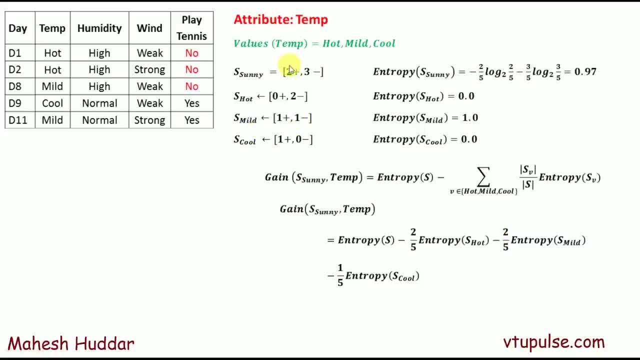 And two examples with respect to mild: out of five, so two by five entropy of S mild. One example with respect to cool, so one by five entropy of S cool. Put this particular formula, put this particular calculated values here. 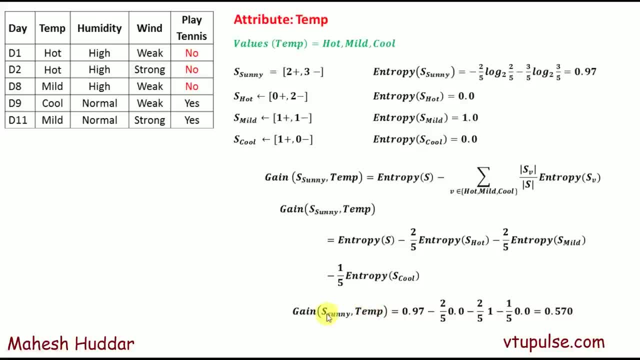 you will get the gain of temperature with respect to S sunny So, which is equivalent to 0.570.. Similarly, we need to calculate the gain of humidity and wind here. So, when it comes to the second one attribute, that is, humidity, 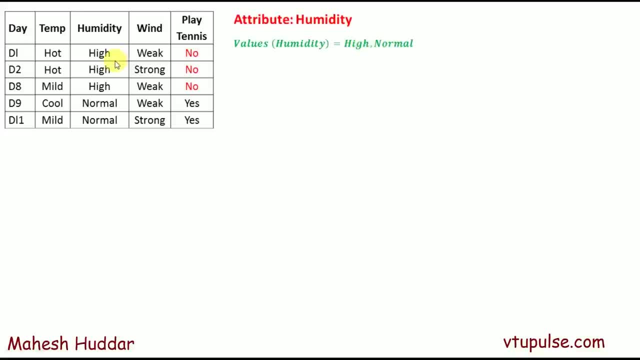 the values are high and normal. There are three high are there and two normal are there, And this is the entropy same for this particular data set. So once you calculate for one attribute, it will be same for the remaining attributes over here. The entropy of S high. 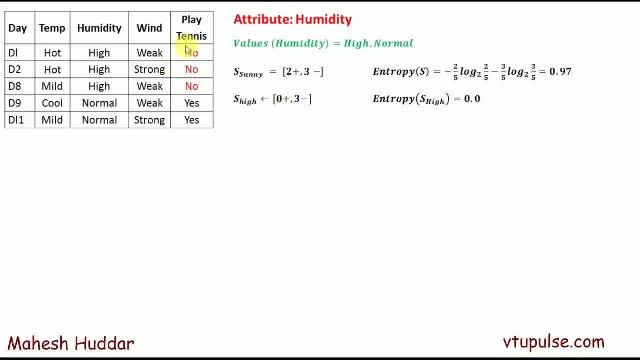 if you want to calculate, there are zero positive examples. are there all three negative examples here, So zero plus three negative, And entropy of S high is equivalent to 0.0 in this case. Similarly, entropy of normal: there are two positive examples are there and zero negative examples. 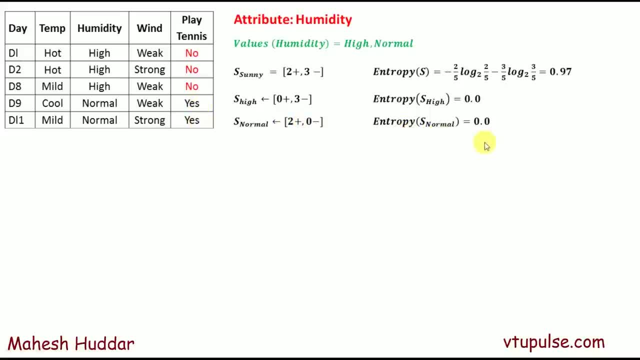 So that is what is written here. Entropy of S normal is equivalent to again zero. And then the gain formula is as simple as that, In this case three by five. entropy of S high, because there are three high examples are there out of five. 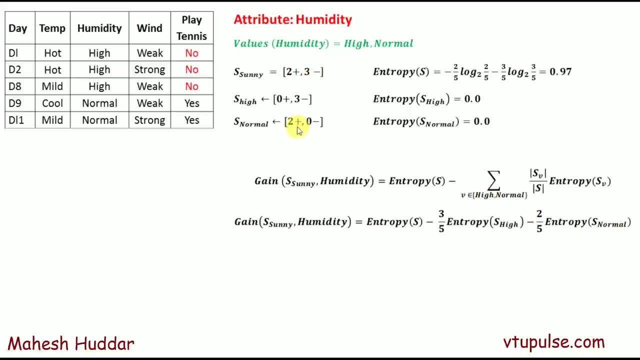 Two by five entropy of S normal, because two normal examples are there out of five here. Put the values, you will get the gain of humidity with respect to S and E, which is equivalent to 0.97. again Similarly, we need to find the gain of wind attribute. 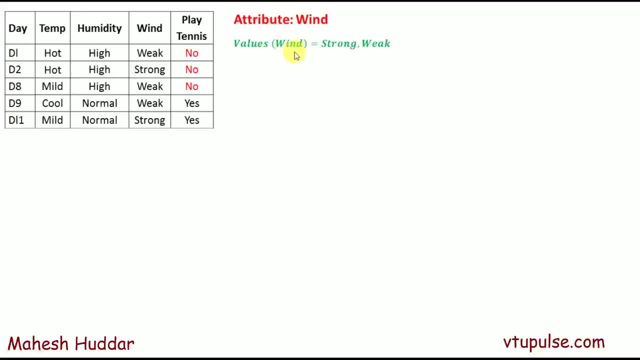 So the attribute name is wind. The possible values of wind are strong and weak. There are three weak examples are there? Out of that, two are negative and one is positive. For strong, one is positive and one negative. So the entropy of S and E is same. Entropy of strong is one positive, one negative, So 1.0.. Entropy of weak is one positive, two negative. Once you calculate it, you will get 0.9183.. So put the values in the gain equation. 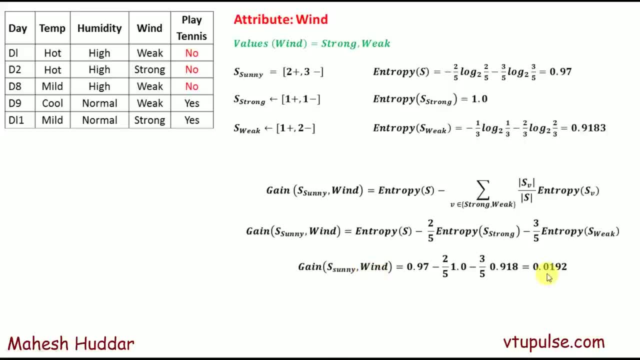 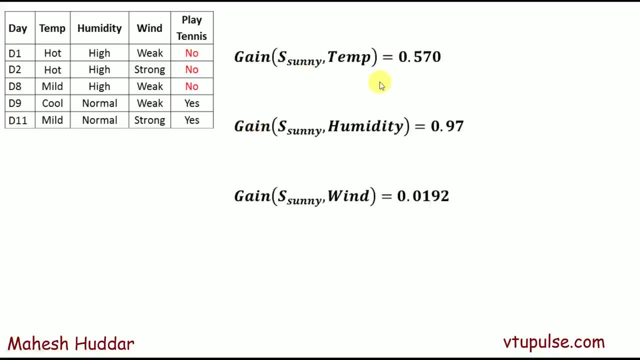 You will get the gain of wind with respect to S and E as 0.01.. Now we list the gain of every attribute. here, Temperature is having 0.570.. We have calculated it. The gain of humidity is 0.97 and the gain of wind is 0.0192. 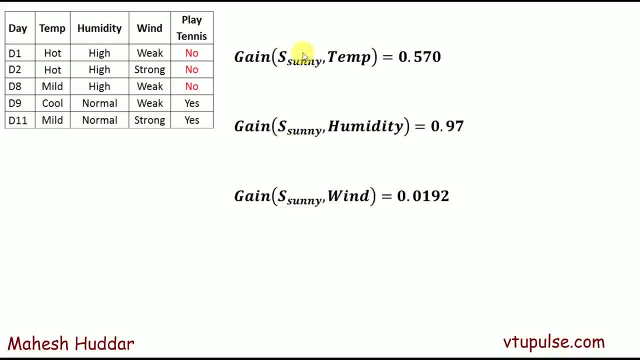 So these are the three things we have calculated. Now, out of these three, the humidity is having the highest information gain. So we consider humidity as the node at this particular level. Now, we consider humidity as the node. There are three. there are two possibilities are there? 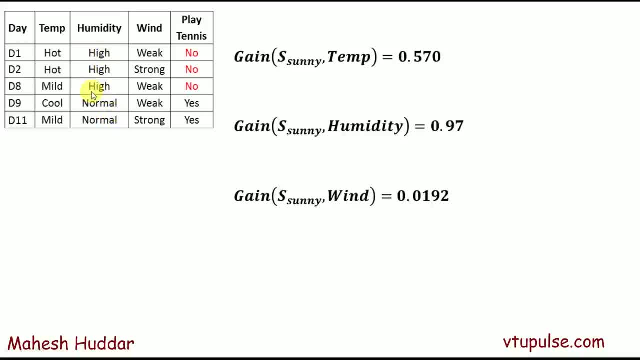 One is high and one is normal. So high is appearing three times and normal is appearing two times: D1, D2, D8 high, D9 and D11 normal. So whenever it is high we have the label as no. 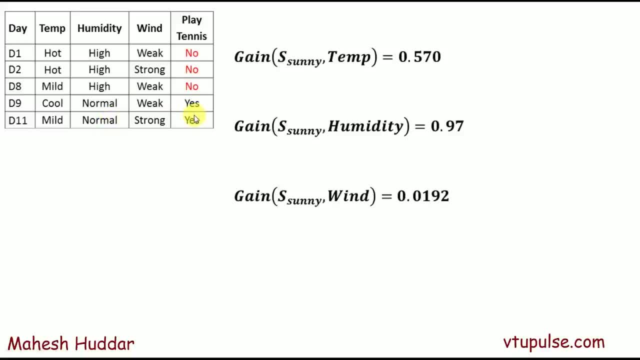 Whenever we have normal, the label is yes. So in all three cases, that is, whenever we have humidity is equivalent to high, we have label no, So directly we can write no here. And for normal we have yes, So we can directly write yes here. 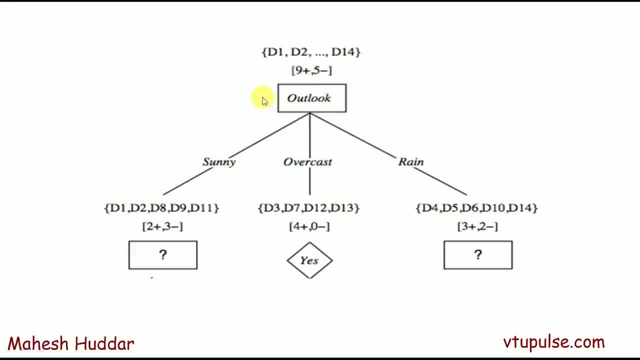 So you can see here, this is what the tree we have drawn in the previous iteration. In this iteration we consider humidity as a node here, Whenever we have high- there are three examples. All of them are no- Whenever we have, humidity is equivalent to normal. 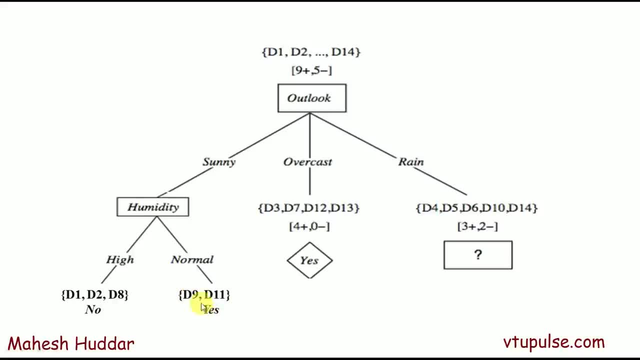 there are two examples and both of them are yes here. So this particular part is over, And this is already over because all of them are positive. So we have written yes here. Now we need to consider these three, Now we need to consider these five examples. 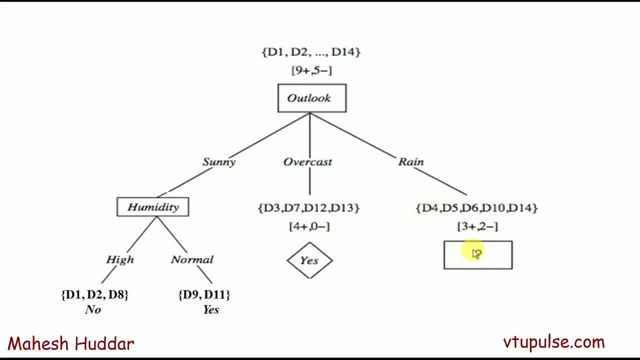 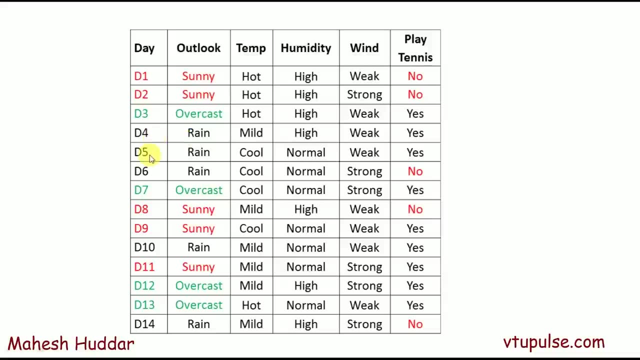 And then we need to consider or we need to calculate which is the node which is having maximum information here Now, from this one, whenever rain is present, that is, D4, D5, D6, D10 and D14. 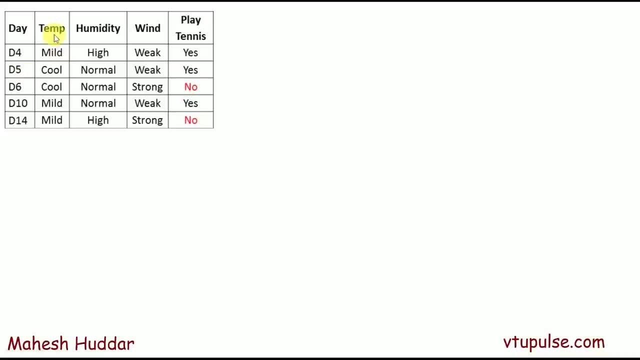 These are the four examples we need to consider. And then again, we have removed that outlook because it is already considered. So these are the three attributes we have on the right hand side. Again, we need to calculate the gain of individual attributes here. 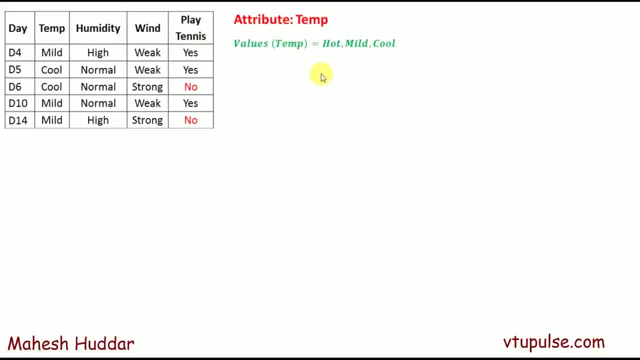 That's the temperature. There are three possibilities again here. Now we need to calculate the information gain of yes, rain here, because the right side, we have rain Whenever outlook is equivalent to rain, we have this particular data set. There are three positive examples are there and two negative. 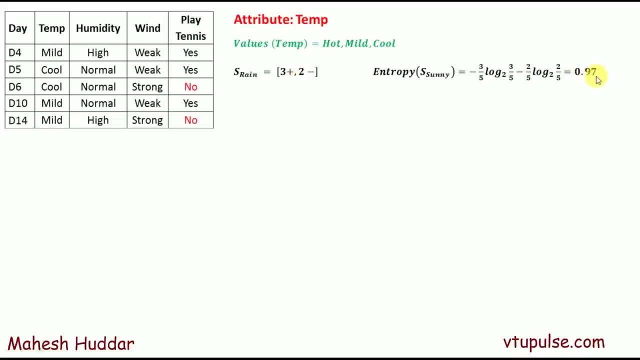 So the entire entropy of entire data set is equivalent to 0.97 here Now the entropy of hot is equivalent to zero. The reason is very simple. We don't have any hot examples. We don't have any hot examples here. So zero positive. 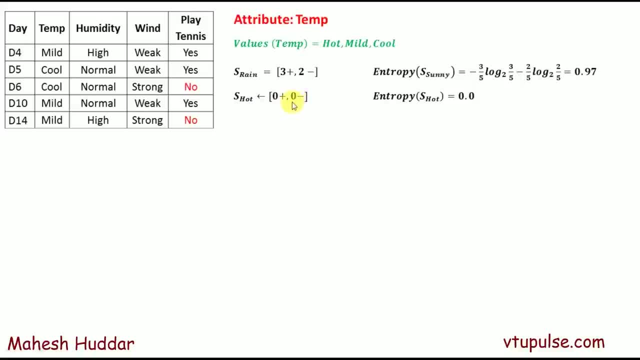 zero negative. Actually, whenever we have equal number of positive and negative examples, we should have written 1.0.. There is one exception for it: Whenever we have zero positive and zero negative examples, we need to write 0.0 as entropy. 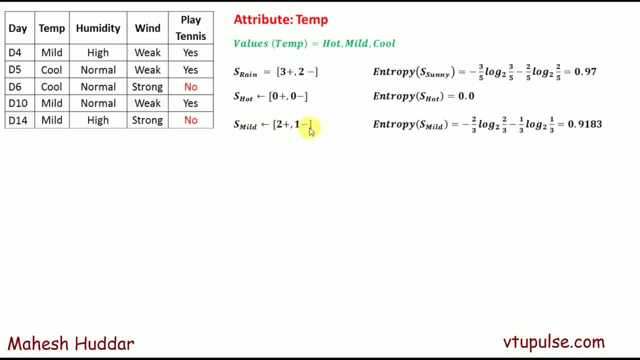 The next one is S mild, Two positive and one negative. we have here One, two, three, three positive, one positive, I think two positive here and then one negative. So the entropy of S mild is equivalent to 0.9183.. 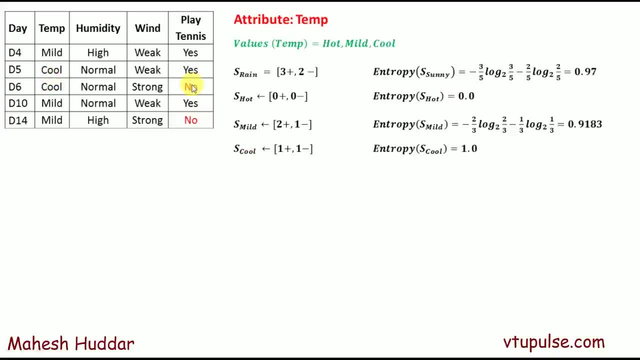 Similarly, the S cool which is appearing two times: one is yes, one is no. So the entropy is equivalent to 1.0.. Put this particular values in gain equation, You will get the gain of temperature with respect to S rain. 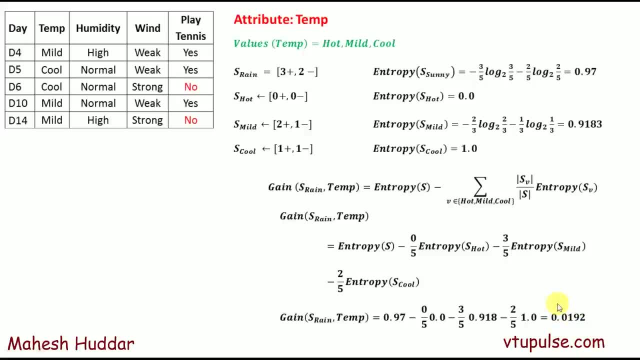 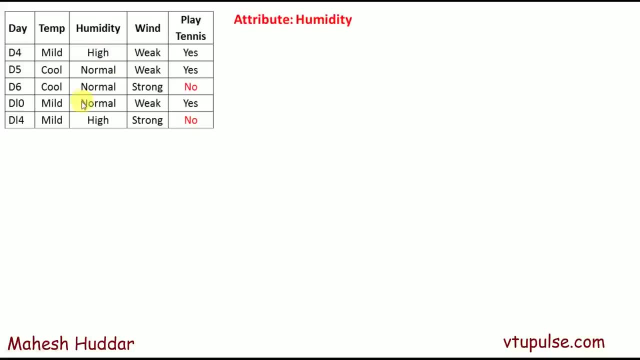 which is equivalent to 0.0192 in this case. Similarly, we need to find the gain of humidity here, That is, it has two possibilities. Again, we are going the same way If we put this value in 0.0 in the gain equation. 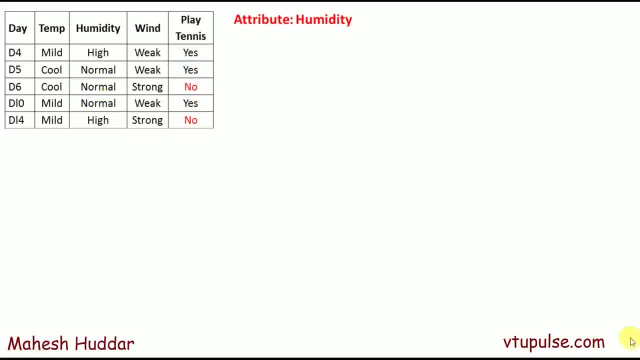 it will get the value of 1.0, 0.0183.. If we put this value in the gain equation, it will get the value of 0.0183.. So I am writing 0, 1, 0,. 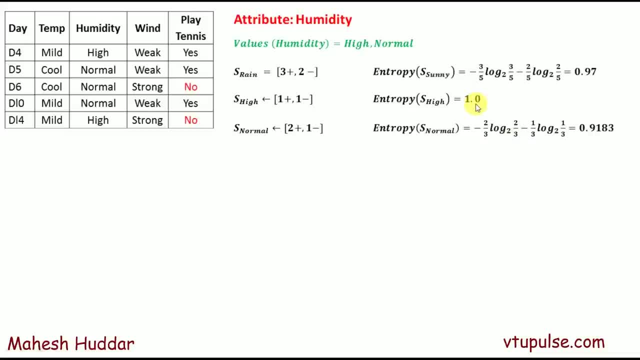 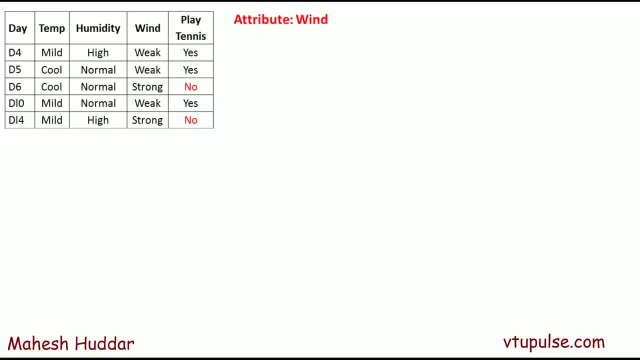 wind. possible values for wind are strong and weak here. so strong is appearing two times, both of them are no and weak is appearing three times. all three are yes in this case. so this is the entropy of fold data set. whenever we have rain as outlook, yes, strong appear. both of them are negative. so 1: 0.0. yes, weak, all three. 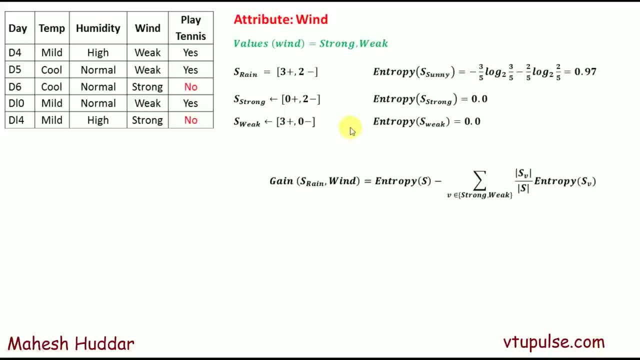 are positive again, N tap is equivalent to 0.0. put these particular values in gain equation you'll get the gain as 0.97 here. so we have calculated the gain of all three attributes. we compare those things. the gain of temperature is 0.019. 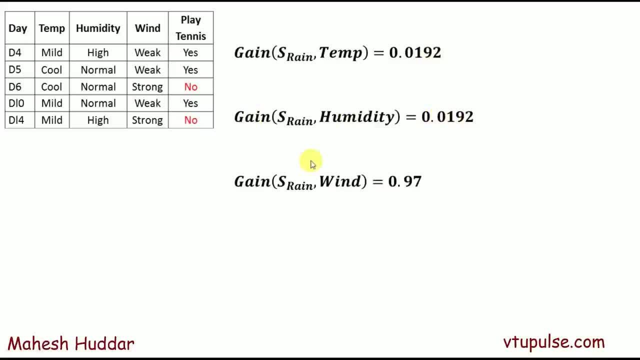 to the gain of humidity is 0.019. to the gain of wind is 0.97. so 0.97 is more compared to these two. so wind will be considered as a node at this particular level. now, if i consider wind as our node, we have two possibilities: weak and strong. Weak is appearing three times, that is. 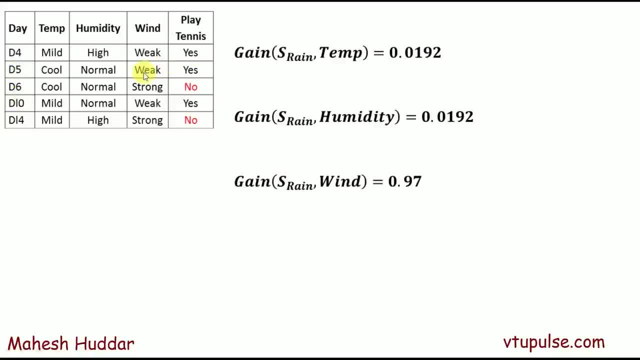 d4, d5 and d10.. In all three cases it has yes, So directly we can write yes, and whenever wind is equivalent to strong- in both the cases it is no only So we will write no directly. So this is. 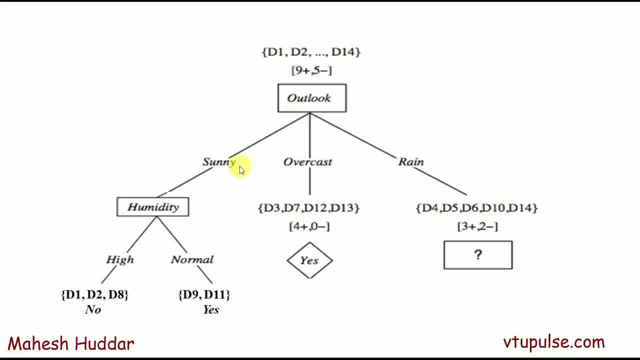 the tree we have drawn in the previous iteration, that is, in the second iteration. For this one, we need to consider wind as the root node. that is the root node we have considered here Whenever it is strong. there are two examples. both of them are no. Whenever wind is weak, there are three examples. 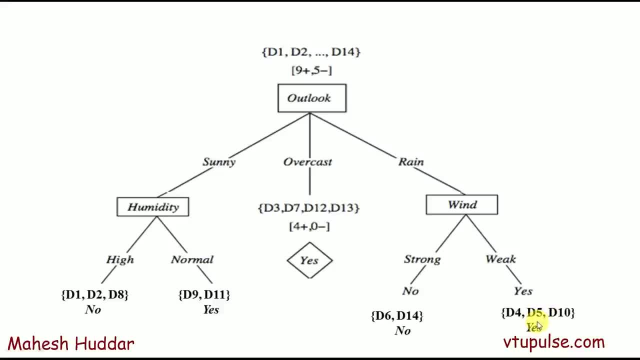 all three of our yes here. So we will write yes directly, So there is no need to further do the further calculation or draw the decision tree. So this is the procedure we need to follow while drawing the decision tree using ID3 algorithm in this case. I hope this particular concept is clear. 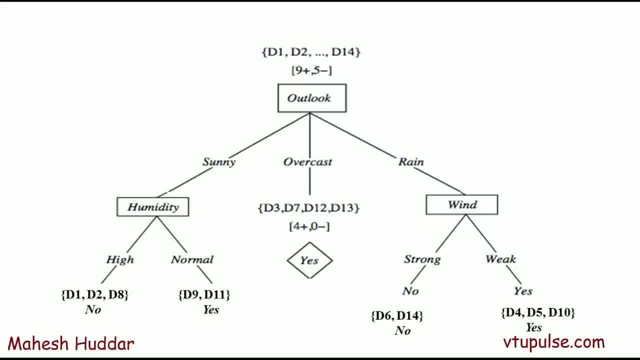 If you like the video, do like and share with your friends. Press the subscribe button for more videos. Press the bell icon for regular updates. Thank you for watching. 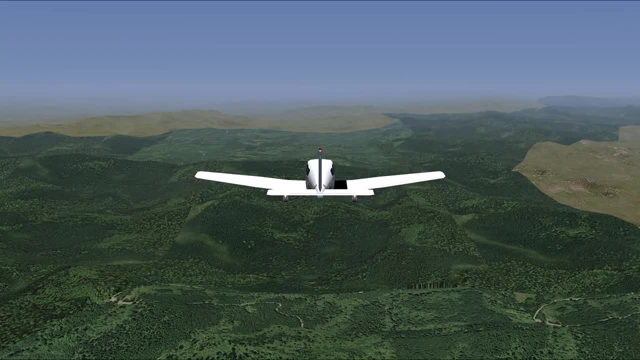 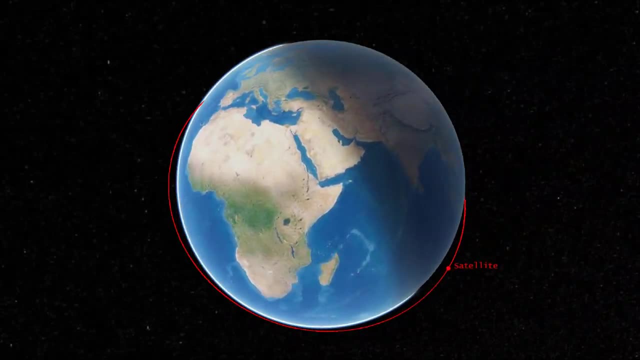 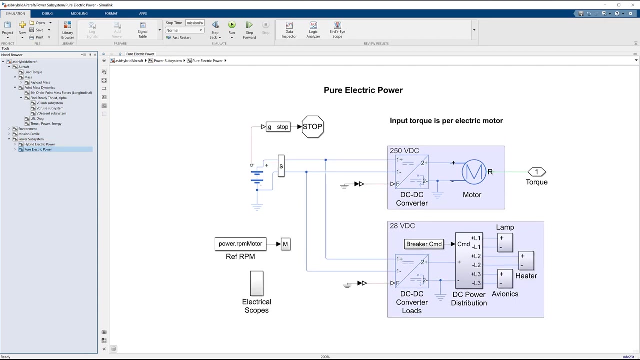 Aerospace Blockset provides simulating blocks that enable you to model aircraft and spacecraft in dynamic environments. implement flight controllers and visualize flight dynamics and orbit trajectories. Start building your vehicle platform models using numerous ready-to-simulate examples, such as the hybrid electric aircraft. 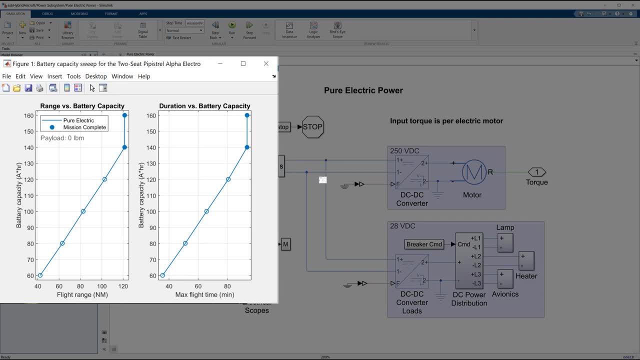 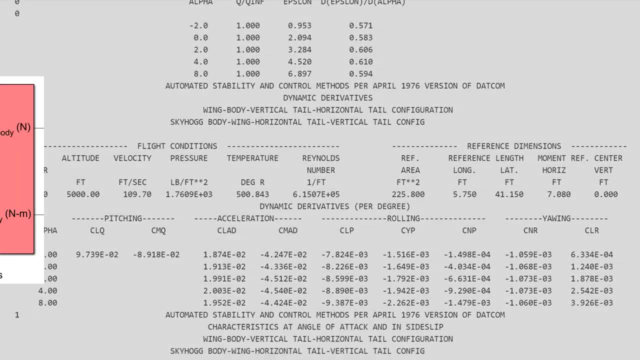 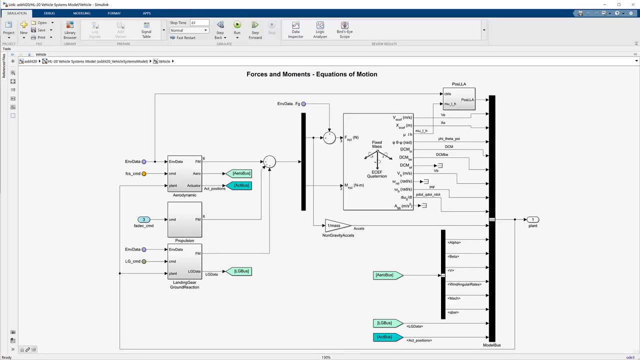 Rapidly explore the design space by performing sweeps on parameters including altitude, payload and battery size. Aerospace Blockset allows you to define fixed-wing vehicle geometries using DATCOM aerodynamic coefficients. You can then use point mass and 3 and 6 degrees of freedom equations of motion to define the vehicle's dynamics. 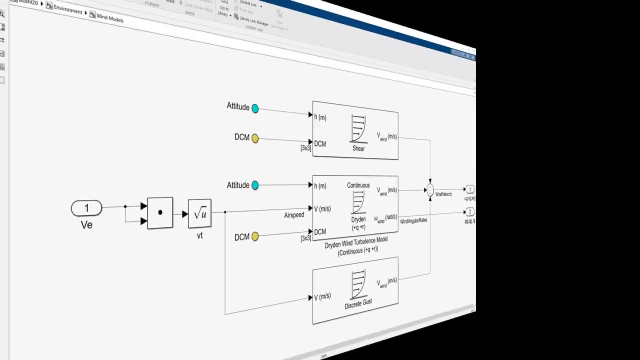 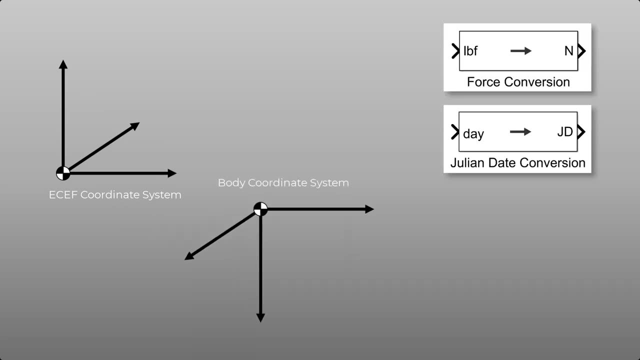 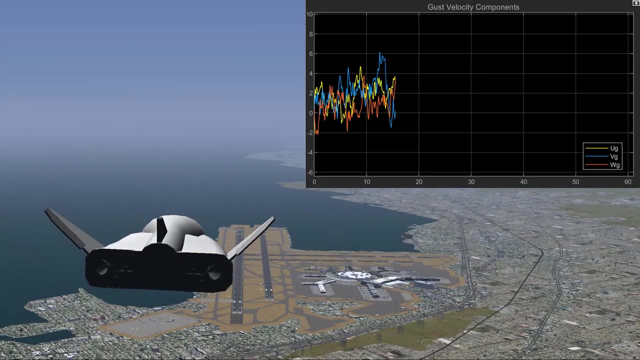 Create higher fidelity simulations by incorporating pilot, atmosphere, gravity and wind models and easily ensure model consistency using coordinate system transformation and unit conversion blocks. Finally, use the FlightCare Flight Simulator Interface to easily render vehicle dynamics and visualize your vehicle in action. 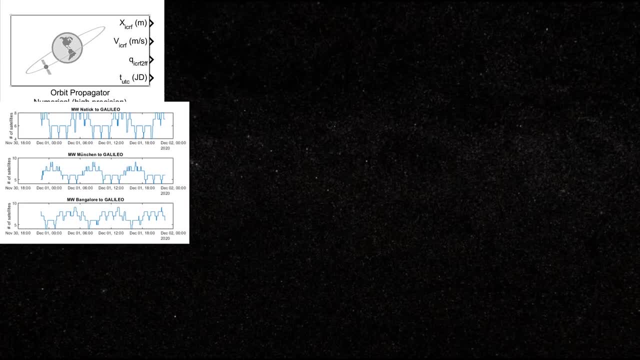 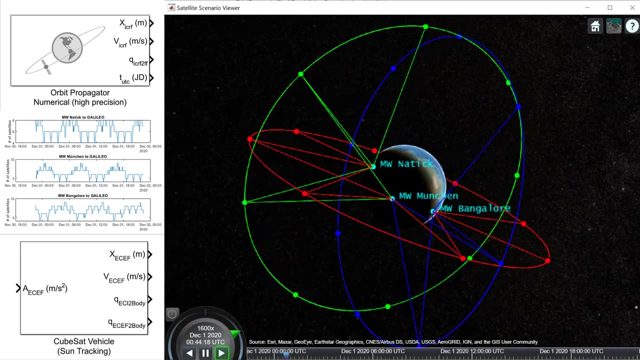 With the Spacecraft Library, you can model the dynamics of spacecraft and small satellites, perform orbit propagation at varying levels of fidelity, compute line-of-sight visibility to ground stations and other spacecraft, and visualize the trajectories and access with the Satellite Scenario Viewer. 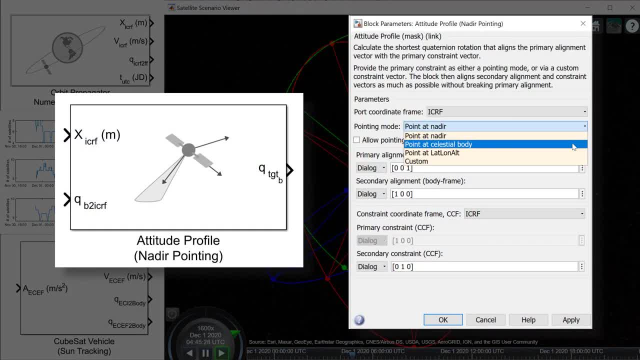 Calculate attitude and control adjustments using Earth Pointing, Sun Tracking and Custom Pointing modes Using the GNC Library. develop GNC algorithms with blocks Using the GNC Library. develop GNC algorithms with blocks Using the GNC Library. develop GNC algorithms with blocks. 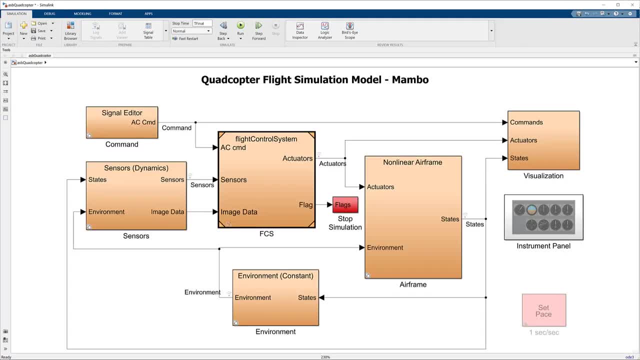 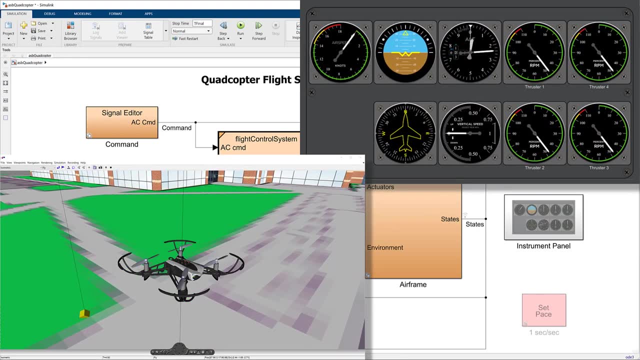 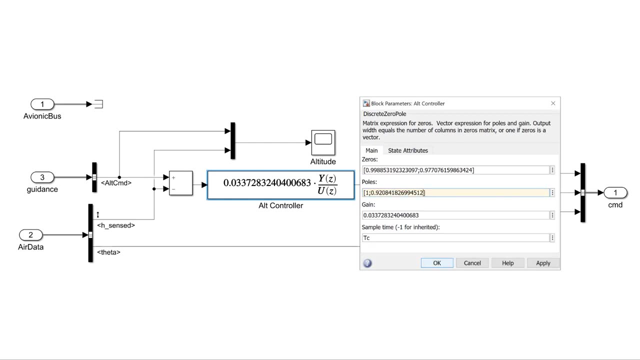 for controllers, navigation and guidance measurements and pilot models. Create your own cockpit instrument panel using flight instrument blocks to visualize signals from your model during simulations. In conjunction with Simulink Control Design and Simulink Realtime, you can tune your controller, test its performance and iterate on the design using hardware-in-the-loop simulations. 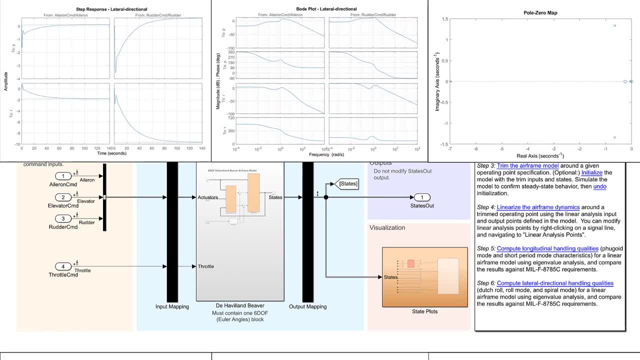 Finally, analyze your vehicle's flight handling qualities using well-known flight standards. Download Aerospace Blockset today to discover new flight handling capabilities. Download Aerospace Blockset today to discover new flight handling capabilities. Download Aerospace Blockset today to discover new flight handling capabilities.